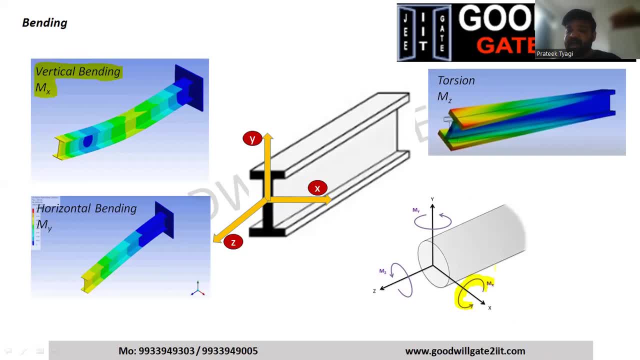 and down. So this MX, if any load is applied, which is known as MX, that will bend my beam in vertical direction. That means it will go up and down. Now next point: if you apply a moment like about Y axis- now you imagine this, don't worry about the direction. 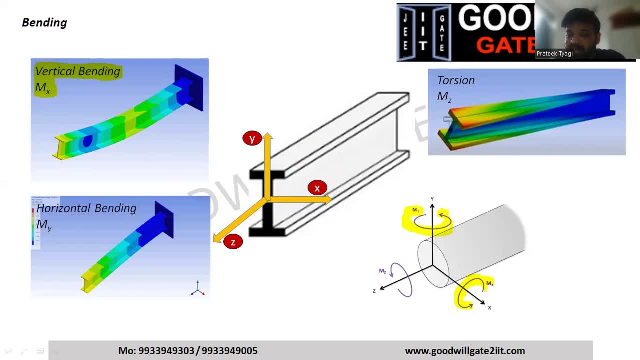 we will see later. If you apply a moment like this, what you're trying to do is you're trying to bend your beam in horizontal direction, And hence this will give rise to horizontal bending. So horizontal bending is one in which your beam move left and right. The moment is applied about. 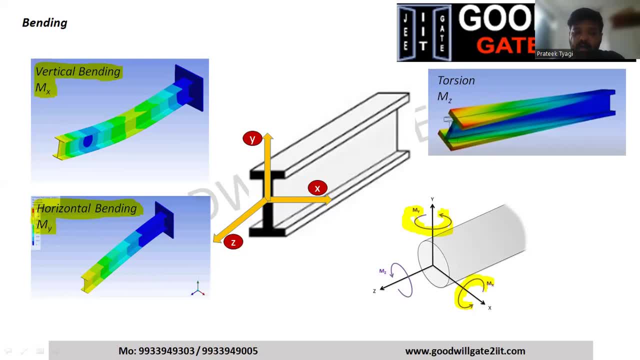 Y axis and hence, just for easy, or just for easy Learning, or just for easily remembering this, we name it as MY. So MY refers to horizontal bending, MX refers to vertical bending. And why MX? Because this moment MX is rolling about X axis. 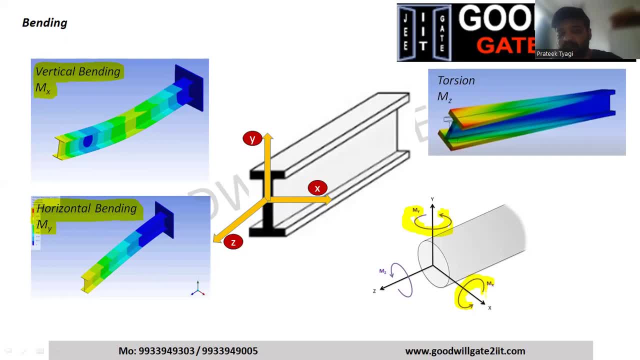 which will give us movement about X axis, means up and down, And if you see why, this will give us movement about Y axis, which will bend my beam in horizontal direction. So you have clear, clear visibility of vertical and horizontal bending. Now, if you people observe this, 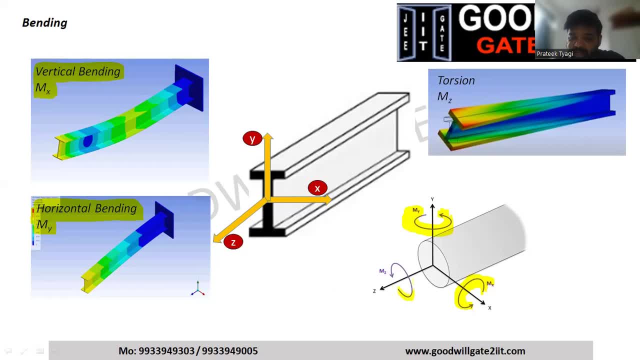 I hope it will be clear. If you apply a moment about Z axis, you imagine something like this will happen. It will twist your system. So, about Z axis, about this axis, about this Z axis, you will be having torsion. So you will calculate all the properties with respect to Z axis. 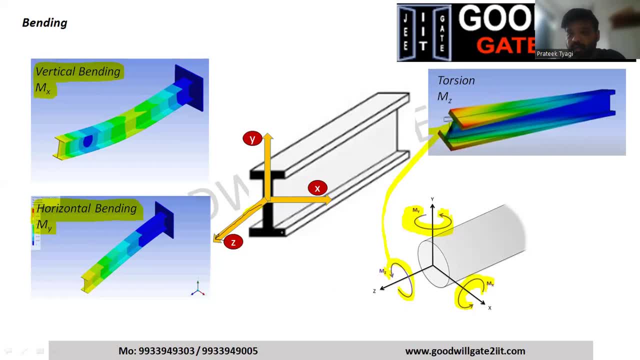 later in torsion. as of now, we are in bending Now. another thing I want you people to understand is if you see movements, because your cross section is in XY plane- I'll repeat this again- because my cross section is in XY plane- I have a movement which is rolling about X axis, So MX. 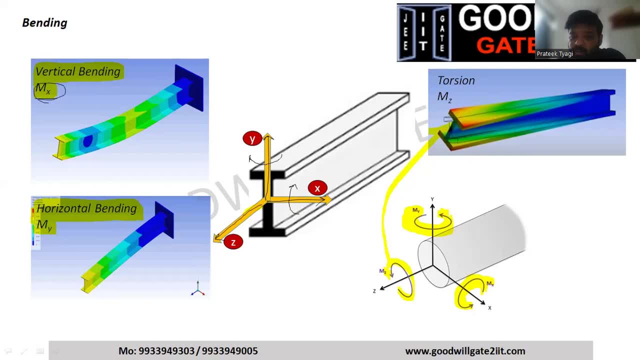 I have a movement which is rolling about Y axis, which is my, so you will not see any mz in bending. mz, which is moment about z axis, which will try to twist my system will come in torsion. so, as of now, we don't have any mz, we will only focus on 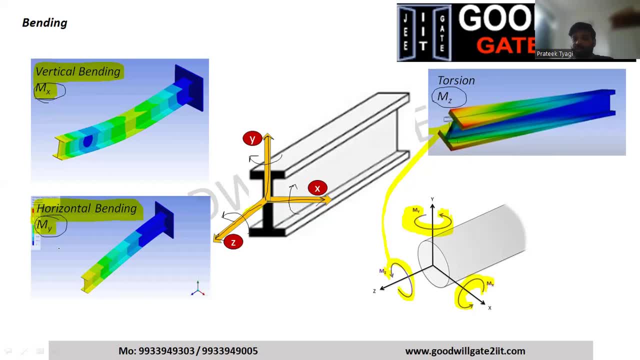 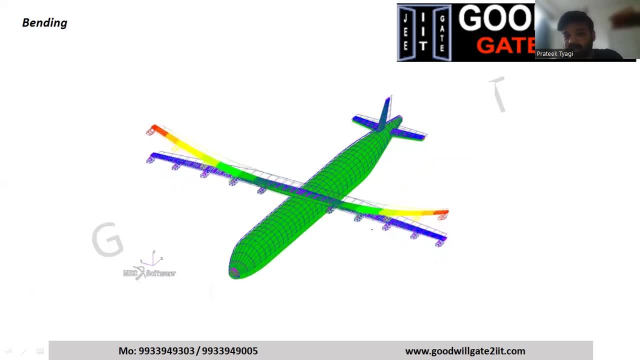 bending, which is mx and my. so i just need a quick nod. and now, why this thing is needed. let me just quickly show you, if you see this right, this is the reason you are studying this in your aircraft syllabus. if you see your aircraft wing, you can clearly observe. that wing is clearly. 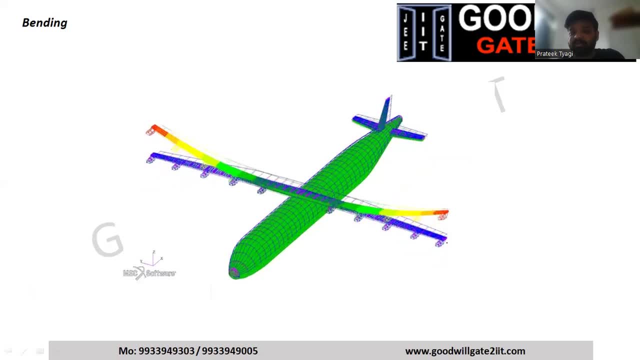 prone or it is very difficult to manage. this is subjected to vertical bending. this is the reason you have cantilever beams, deflection problems, stress calculations in your syllabus. so i hope this is very, very much clear to you people: what is bending, what is cross-section, what is xyz? 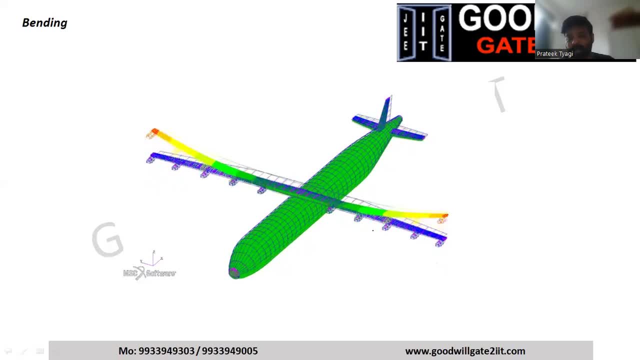 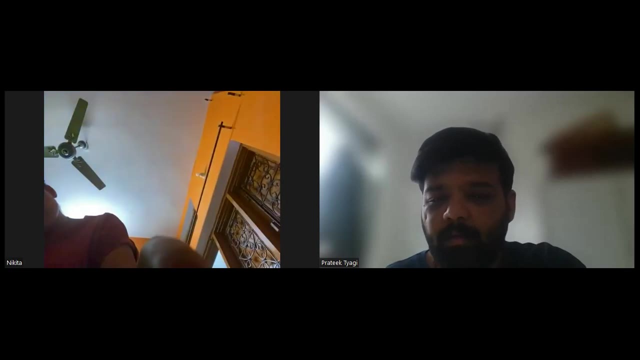 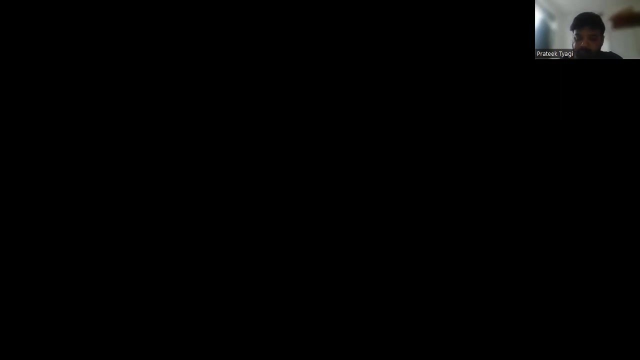 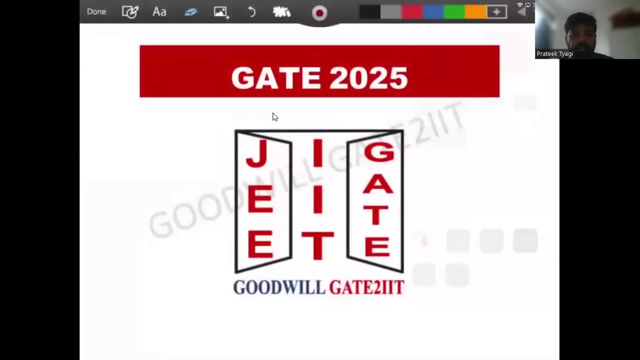 coordinate system. and if it all this is clear, then i'll go back to my uh presentation mode and i will start developing equations on this. is this clear for everyone, guys? okay, okay, now i am back to my presentation so that i can develop equations. i have framed this lecture completely, even if you don't know. 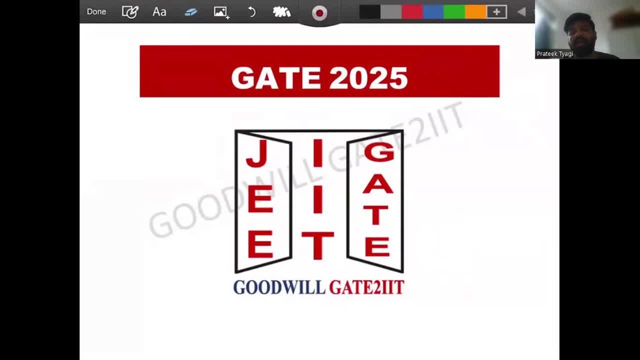 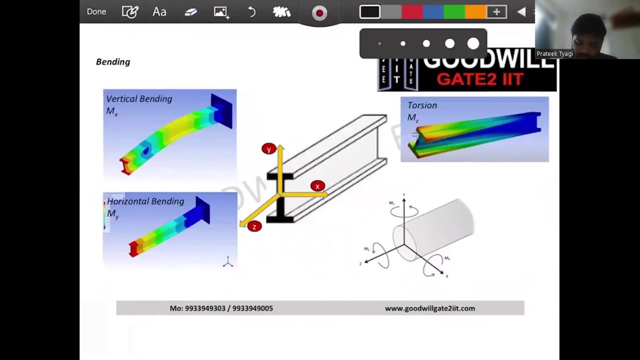 anything about bending. by the end of this, you should be in a position to solve any numerical or any- uh, difficult questions which comes for bending. all right, let's solve this now. okay, perfect, okay. so this is the slide which i have already shared, so there is no difficulty in this. 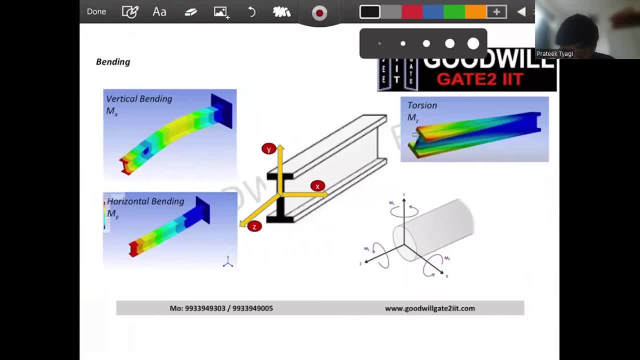 this is the reason i was saying: if you apply a movement about x axis, you will be able to solve any numerical or any numerical problem. so you are simply trying to make beam up and down, which is vertical bending. if you apply a movement about y axis, that means you just try to make your beam go. 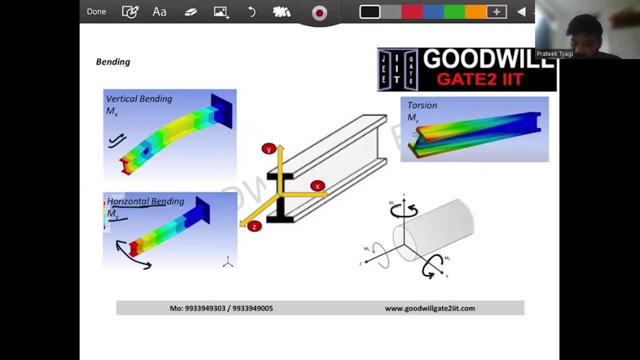 left and right. this is horizontal bending, and if you apply a movement about z axis, in simple words, you are trying to apply a movement like this which is about z axis- this is your z axis right, so you will twist your beam, which is altogether a separate unit. now let's go to our equation. 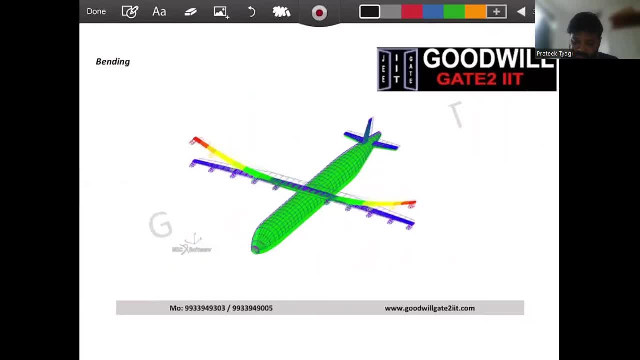 which is very, very difficult equation when we go to mexen and this is your aircraft application. you have already seen this: this beam, this is the cantilever beam which is fixed here and, if you see, this beam is bending up. so this up and down is nothing but vertical bending, but we're not going. 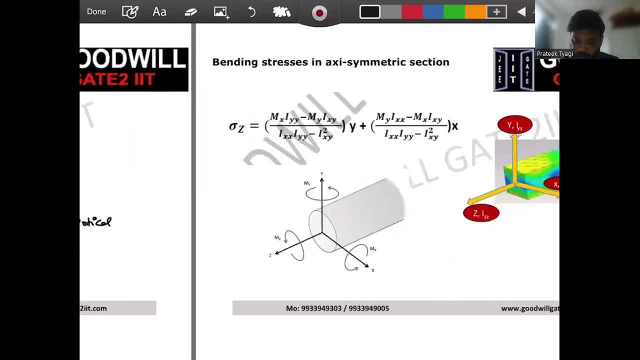 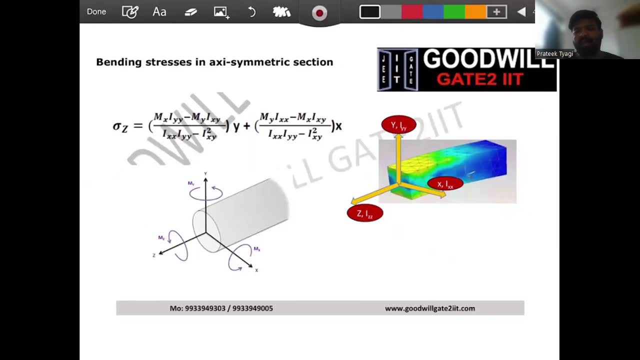 to study only vertical. we will see both horizontal and vertical. now i'm coming to a very difficult equation, but believe me, i will try to make it simple for you so that we can solve any human gate. numericals are very simple, instead forward based. that is not my concern. the concern is: sometimes they ask a difficult 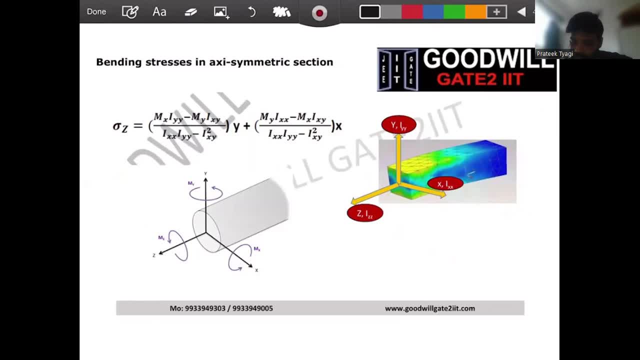 question combining bending torsion and all these questions. so let's go slow in this. so if you see, this is the length of the beam, please focus very hard for next 10 minutes so that you can understand this equation. this is the length of the beam. it may be fixed somewhere and if you 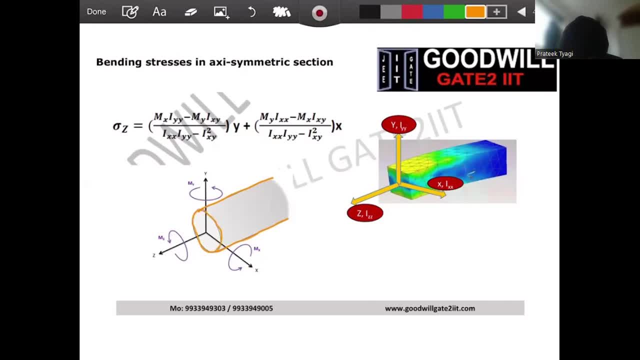 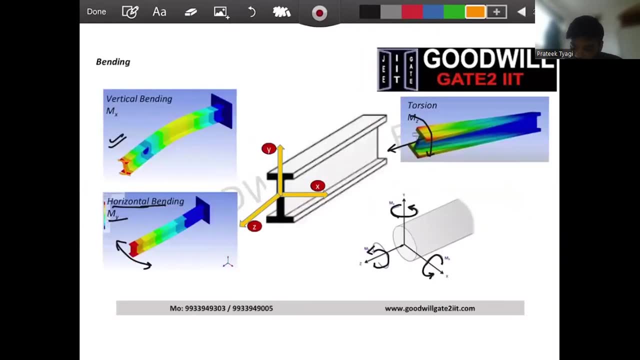 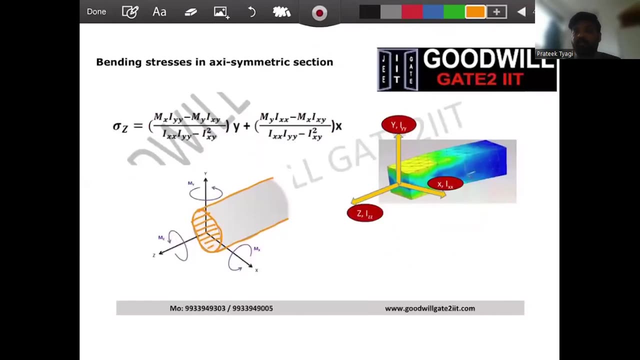 see, this is my cross section. all right, this is the cross section of this beam. here you have seen cross section, as i you. here you have. i'm just giving you an example with circle and then you can have rectangle, you can have c section, anything. now you are clear what section. 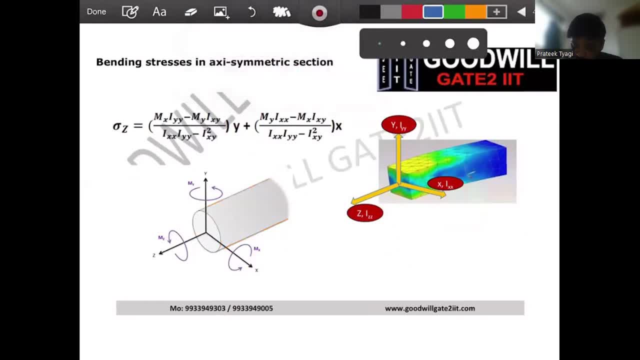 means now in this cross section. if you people see, this is my x-axis, please, please listen to me very carefully. if you see, i have taken another example in which my cross section is rectangle. here my cross-section is circular. any shape i don't bother. then this is the x-axis. now i want you people to be clear in. 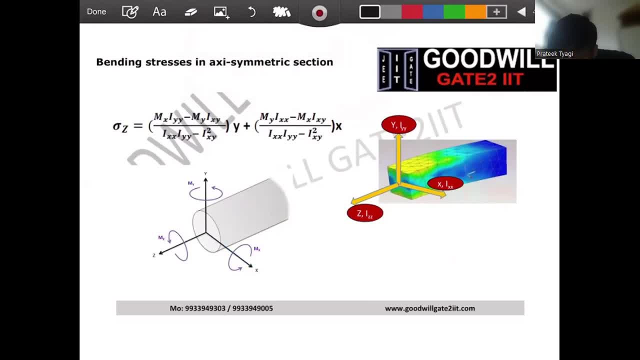 this: when i say x-axis at this point, we will see this is centroidal axis. x is 0 here. at this point, if let's say this dimension is 10, you will say x here is 5 and you will say x here is minus 5.. i hope this is clear. everyone understood what is minus 5, what is plus 5, because total end is 10.. 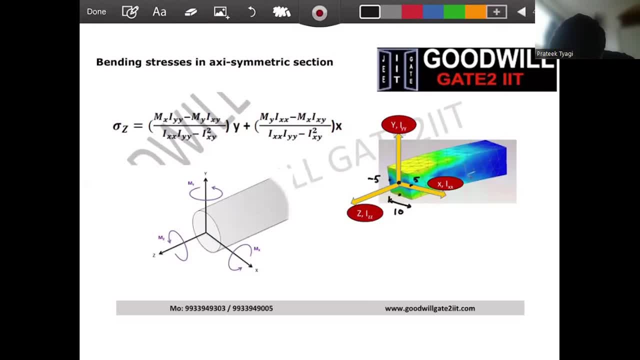 similarly, if you go here, you will say this is minus y, this is plus y. and similarly, if you go to this point, you will say: this is x 5 and let's say y 5. so this coordinate is 5 comma 5.. so this: 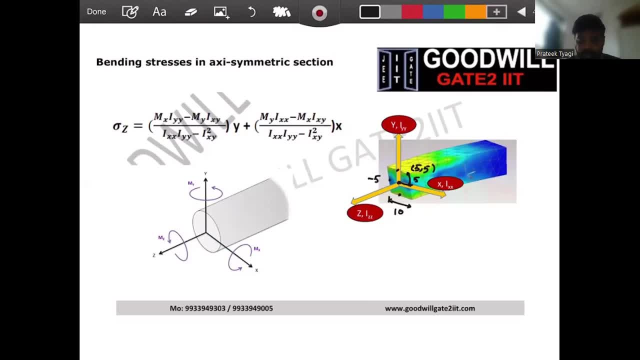 is how cross section varies in x- y plane. all right, first thing, i want you people to be very much clear. you will say: calculate the maximum stress, calculate the stress at this point, blah, blah, blah. many numericals will come right now. what next thing to understand here if you have a movement about x-axis? 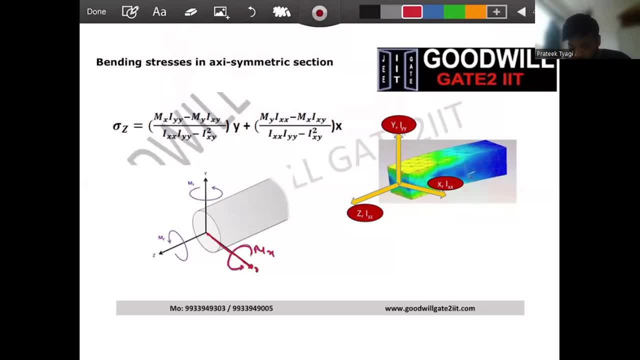 which is mx. so you are rolling about x-axis, so the inertia about x-axis will be calculated now. i will do all today for inertia. how to calculate for circle, rectangle c, i, z, any cross section. we will solve everything today. but what i'm saying is when you have x-axis, mx and you know this is vertical. 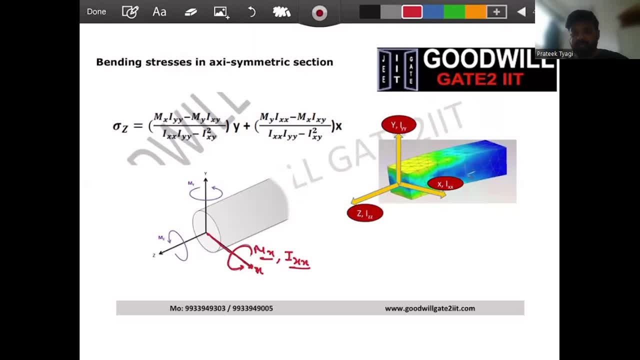 bending, the inertia will be about x-axis, which we name it as ixx. i will give you the properties in some time. so if you see i have written it here, if you are rolling anything about x-axis, the moment is mx and inertia is ixx. then if you roll anything about y-axis, your moment is my. 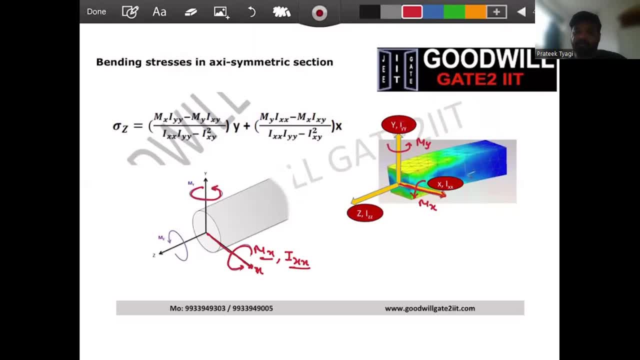 and inertia will be iui, and if you rotate anything about z-axis, your moment will be mz, which typically we write it as torque t, don't worry about it- and your inertia is z. so you have three inertias: ixx, iui, izz and you have three moments: mx, my mz, but 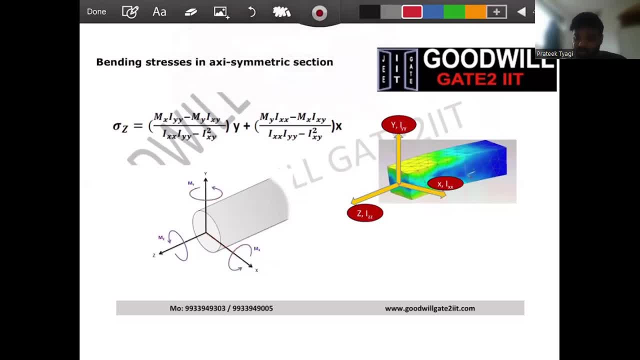 if you people see, bending will only happen because of two people: mx and because of my- forget about mz for now. so we will not bother about this axis because i am not interested in twist of the section, i'm only interested in bending of the section. so if you clearly observe this bending equation right, i explain you what. 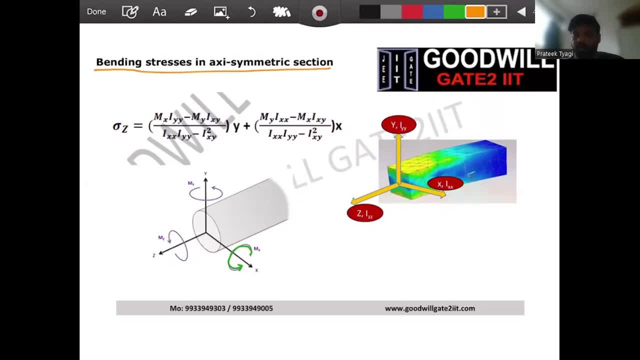 is axis symmetric? what is symmetric? in few minutes, no, no, no, buckling is entirely different. please don't get into it. i will come to that. so if you see your right hand side equation right, first thing you observe here is that you have two brackets: one is with y and the other one is x. 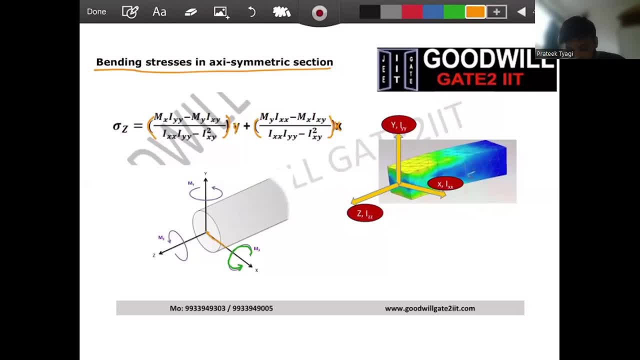 because your cross section is in x and y plane. if you see, your cross section is in xy plane and the moment which you can apply are only mx and my. so what i want you people to see in this equation is: this is easy to learn. now, because your cross section is in xy plane, you have 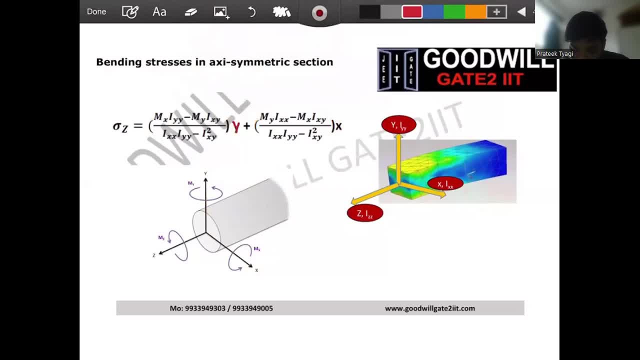 two brackets here. one is y this term and another one is with x this term. and if you see the loads, loads in the sense moments, you see there is only mx and my. there is no concept of mz here. so you will not see mz throughout your bending. there is no mz concept. 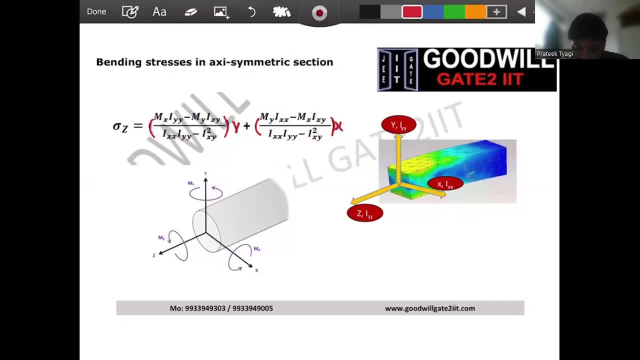 there is no z axis we were worrying about. so if you see m x, m y, m, y, m x, don't worry about why it is where. as of now, we just need to learn that there are movements present, which is mx and my, all right now. next, so this: 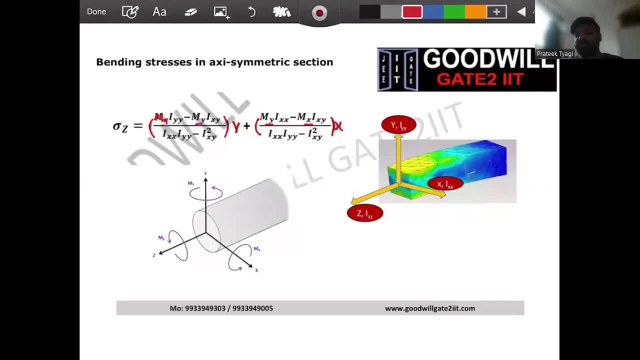 is somewhat clear now: when we have x axis, when we have y axis, when we have movement mx, when we have movement my, the inertias will be i, x, x, i, y, y and we will learn slowly: i, x, y. but if you see, the entire equation on right hand side, right is only in terms of x and y and y, because your 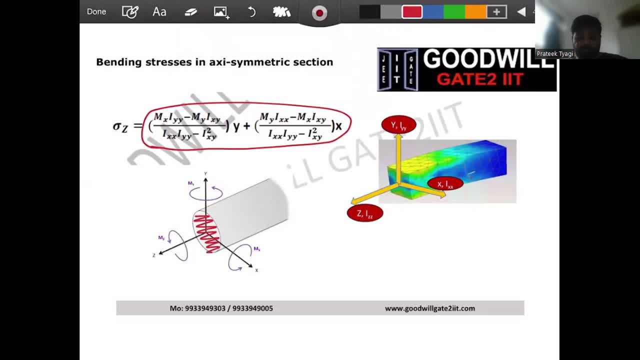 cross section is in x- y plane. this is both one thing which should be crystal clear to everyone. what do you mean by this equation? i will tell you what a sigma z later, but as of now, is this clear for everyone by this whole equation on right hand side, if you observe. 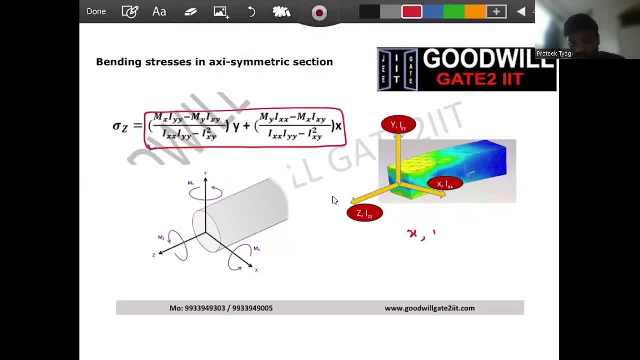 is completely in x, y. you see, it has xy terms, it has mx, my and it has all the inertias about xy plane. don't worry, what do you mean by these quantities? i don't expect you to know this least. you should know, in this bad equation, everything on the right hand. 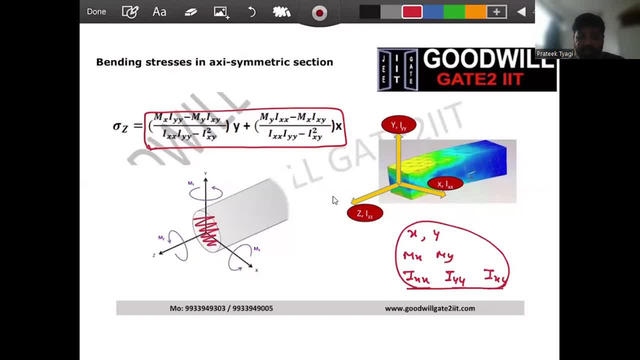 side is in XY because your cross-section is in XY plane. Give me a quick nod. if this is clear for everyone, then I will go ahead. Is this okay? Clear for everyone? Anything, any doubt, any misconception you want me to repeat? just let me know I can. 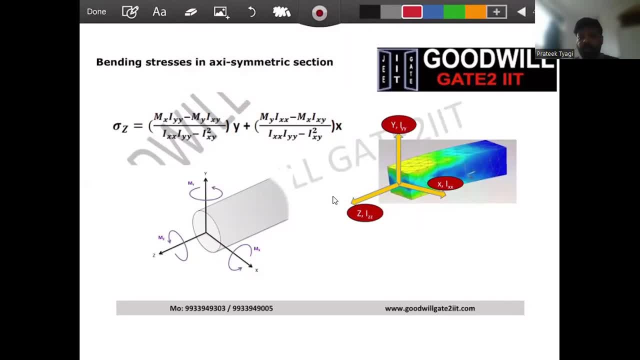 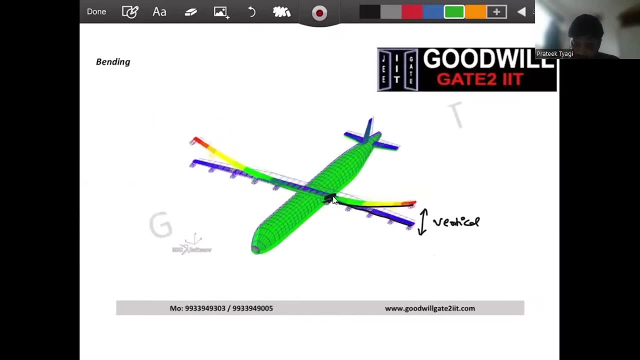 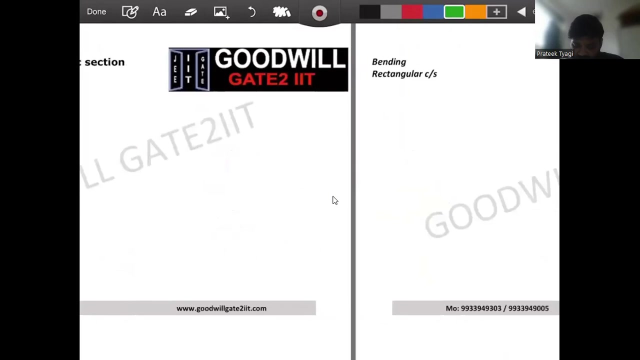 give in detail. All right now, let's see what this Sigma Z tells. I don't know whether I have kept an image. no, okay, still, I can explain you that All right now. see what happens when you have a beam. right, I think I've kept some image. 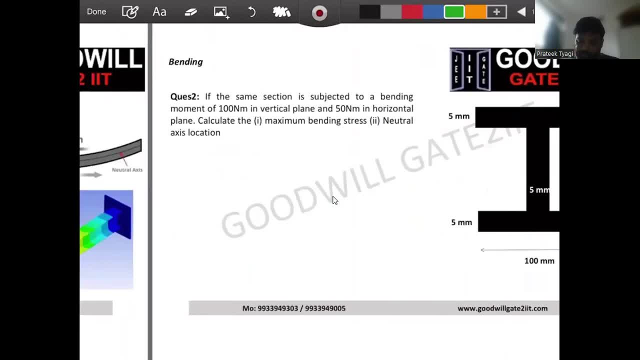 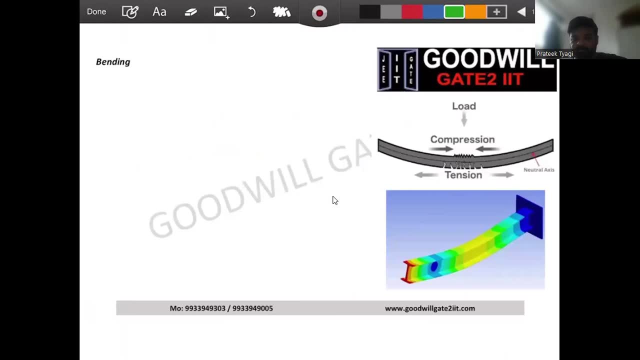 I think, yeah, I can show it from here. Okay, Please listen to this carefully, what I'm trying to explain here. Any cross-section, Akash, your cross-section is in X&Y plane. The bending is not occurring in XY plane. I told you right, you have. 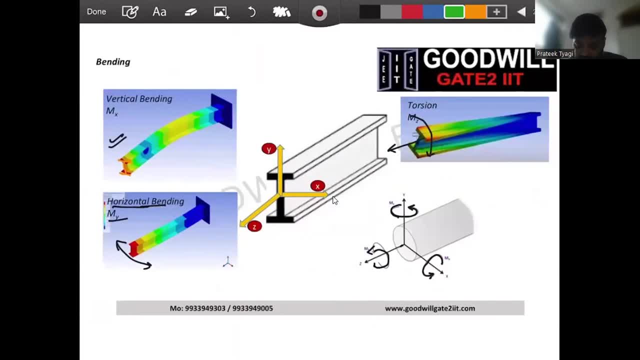 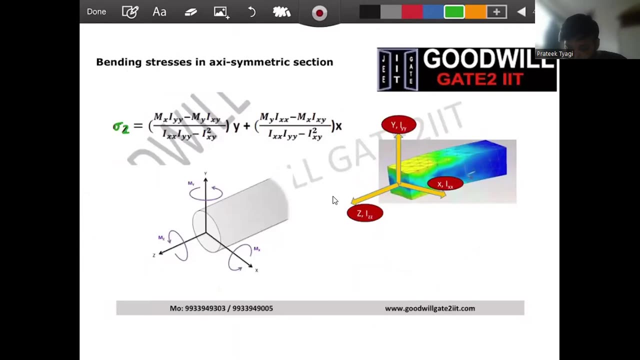 assumed your cross-section is in XY plane. See, this is X and this is Y. This is X and this is Y. This is your cross-section, right? This is: this is X, This is X and this is Y. So your cross-section is in XY Plane. Plane is 2D, right? 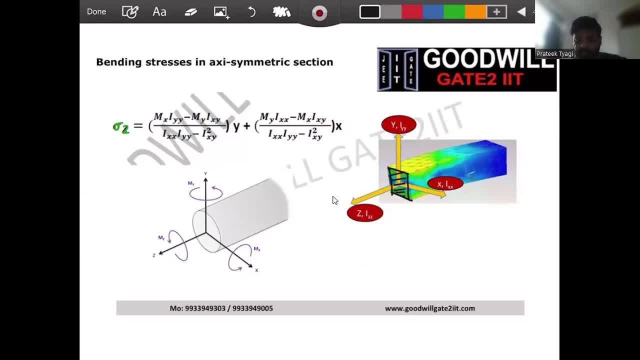 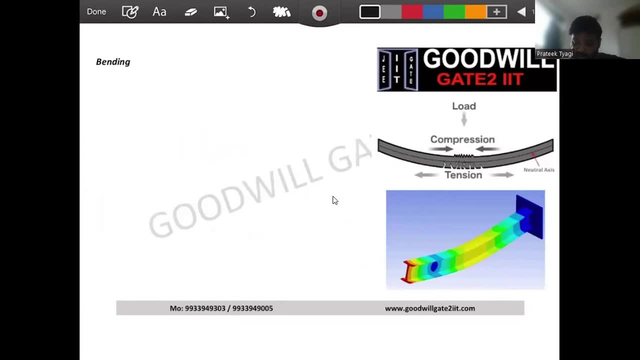 Clear Akash. Yeah, Now guys, I want you to understand one thing before going into that equation and start solving some numericals: When you bend a beam, right, You can see. this is what you see in thisефine Trinity: V dot X, right? This is the kind of transductions that shall. 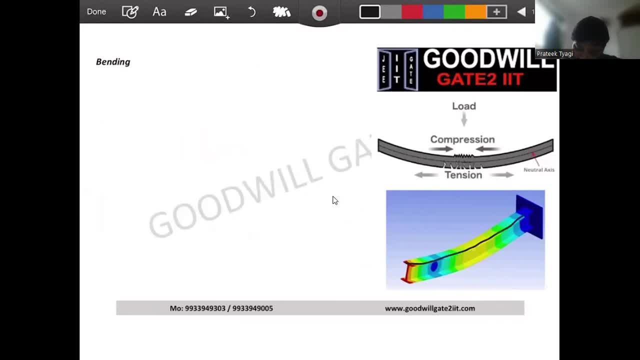 happen, Change your approach and either curves or curves or anything else of that nature. I won't talk too much about it for now. Thanks, kakash, Bye, Okay, Bye, bye, Bye. bending right, this beam is going up and down. So if you see it from this end, if 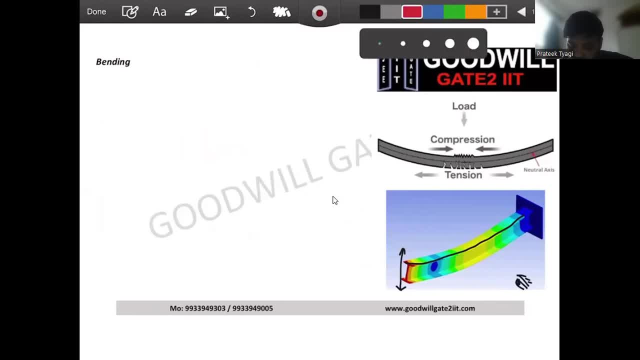 you see it from this end, you will see something like this, which I have drawn this diagram. If you see what happens here on the upper section, this section, you are compressing it. You can imagine this in your mind. and if you see this, 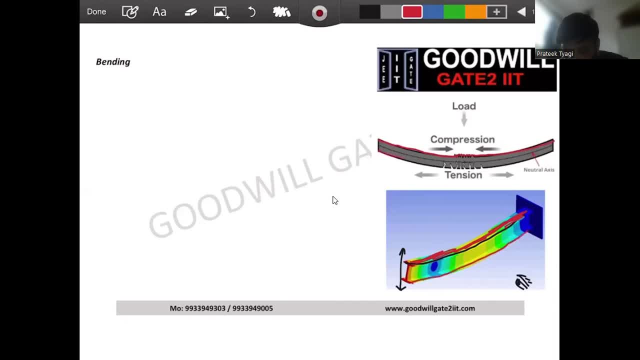 below section right, this section. this is in tension. you can see what will happen. and if you keep on bending this right, what happens? this system will break from center. It will be divided into two sticks, two pieces. Now, with this, what I'm 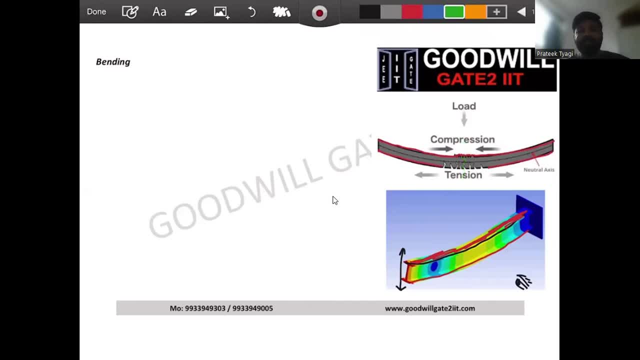 trying to explain you here is when you bend a beam, right when you bend a beam, the stresses which are known as bending stresses are generated. Now, when you bend a beam, the stresses which are known as bending stresses are generated, and these bending stresses are nothing but normal stresses, which acts perpendicular to. 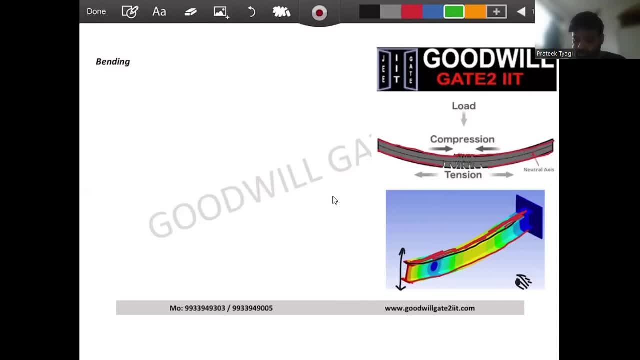 cross-section. now imagine or visualize this in layman terms: when you bend any system right, what ideally beam experiences? as if someone is pulling me in this direction and this direction as if someone is pulling me, although you are not pulling this. you are bending the beam, but 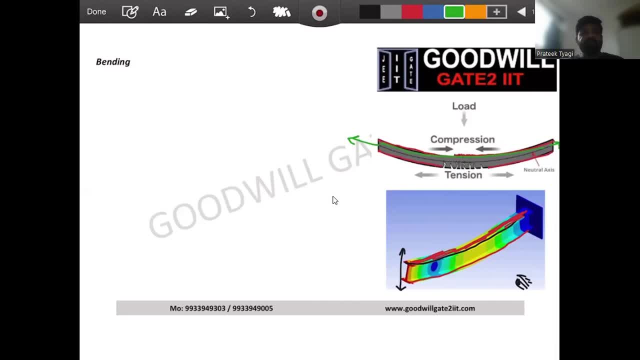 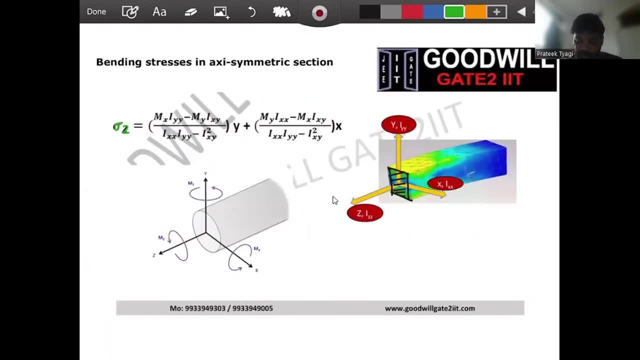 structural experience is as if someone is pulling me in this direction. now, what do you mean by this? let me make it more clear. when you have any beam like this and you bend it by any amount, i'm not interested in which direction you're bending it. so what happens? 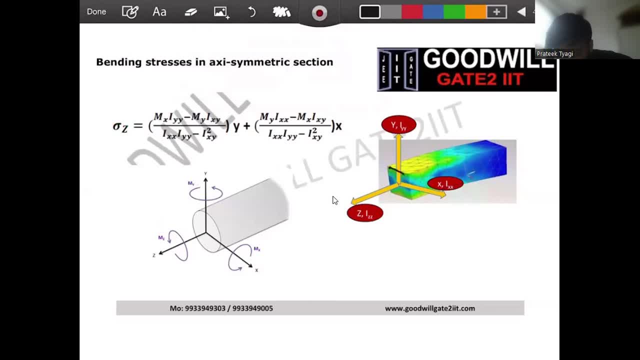 is, guys, please listen to me carefully. it's cross-section experiences, normal stresses, which is represented as sigma z, and similarly there will be stresses here. now, what is a normal stress? a normal stress is one which is perpendicular to cross-section, correct? what is the cross-section variables? if you people 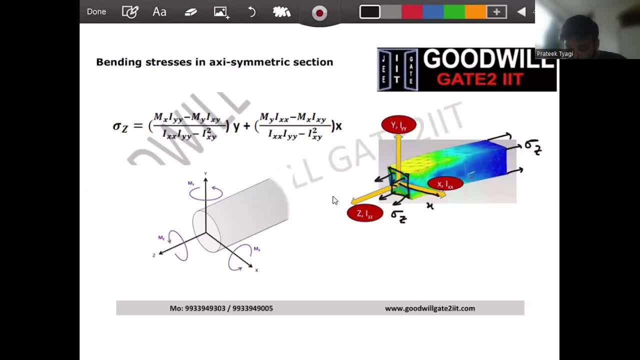 agree. your cross-section is in xy plane, so anything which is perpendicular to it will be z correct, and this is the reason you find sigma. sigma here represents normal stresses going in z direction. so, guys, what i am simply explaining you is: if you have your cross section in xy plane, if this is x and this is y, that means you have movements: mx and my. 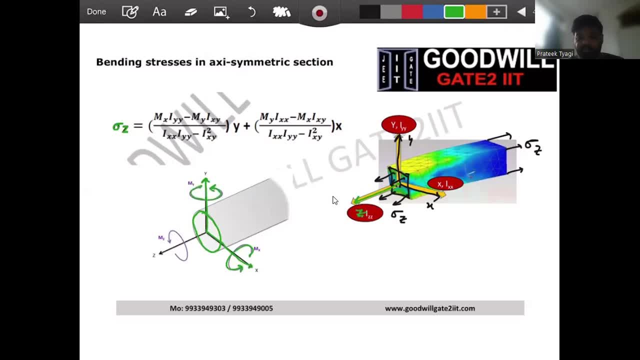 and if you apply these movements, you will get stresses which are perpendicular to it, going in z direction, and hence you have sigma z. This is the most beautiful equation which is present in mx, and you must have seen this in your academics. if not perfectly fine, you will. 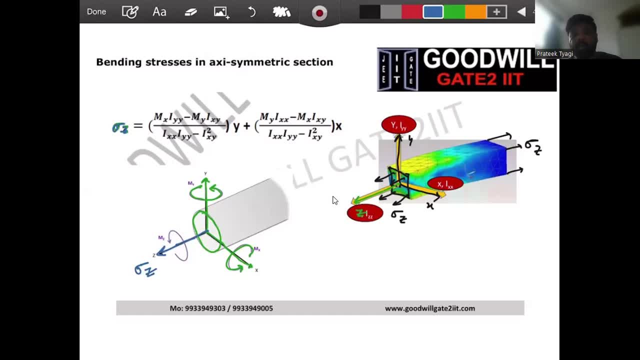 be doing this in your maybe third year or something, but I hope everything at least. learning formula is different, but at least you people understood that. what do you mean by this sigma z? This sigma z are nothing but your bending stresses. Bending stresses means the stresses. 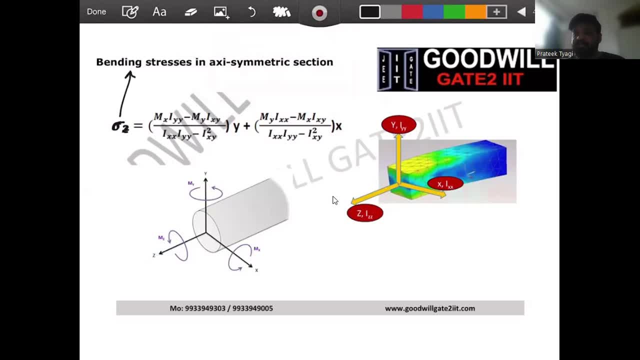 which is coming because of bending. What are these stresses? These stresses are nothing but stresses which are perpendicular to cross section. Now question in your gait exam they will ask is: what is the maximum bending stress and where it occurs? So stresses acts on complete cross section. Your stresses act here, here, here, here, here, here. 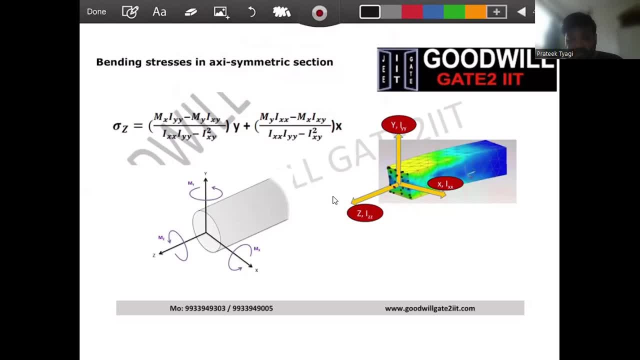 here, Everywhere in cross section, stresses are acting. All these stresses are perpendicular to cross section, as if you are trying to pull this beam Out of all this in your cross section. where is the maximum bending? stress is what your gait numericals are and your complete 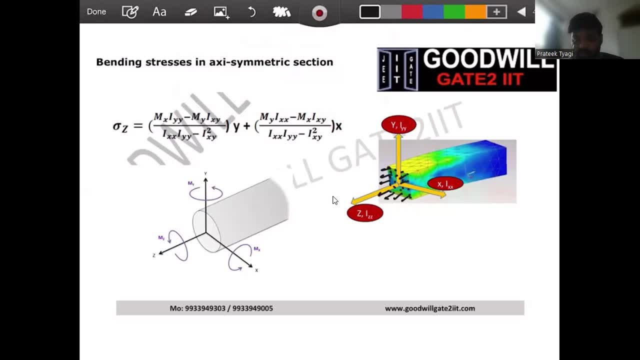 max and also so on. this, Any exercise, or solid examples. if you see right, you will be talking about this maximum bending stress, which will be calculated using this formula. Now I want to go one step further. The next thing we need to understand is, first of all, how we learn this formula. all right, Let me give you a hint. So what I do is: or you, 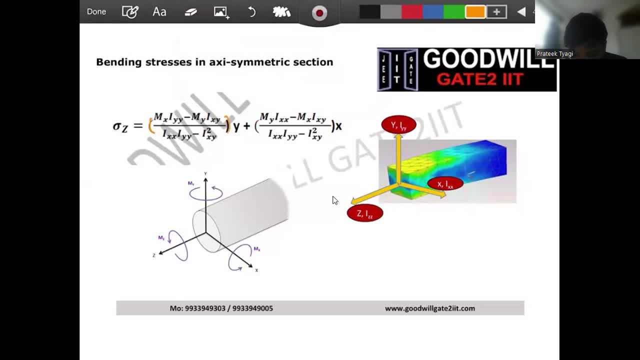 typically try to follow this formula. So you typically try to follow this formula. So you this: you write two terms as this, Y and X. because your cross-section is in XY, you write in this way: then you, in both the terms, you write your denominator like: 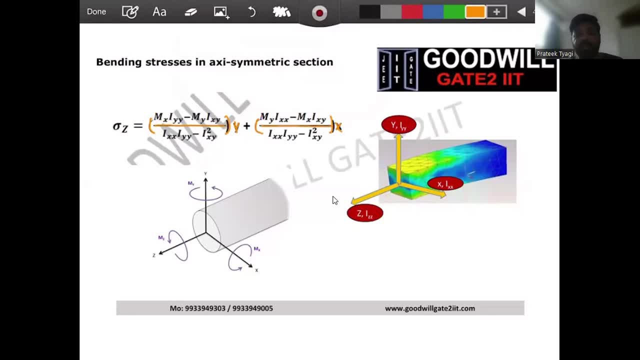 this: IXX, IYY minus I square XY. I'm telling you how you should remember this, because this is asked completely in your GATE exam. so you calculate, you just write these terms. then, once you see Yher, you first right your IYY. you see X, here you write IXX, like then, once you have written IYY. 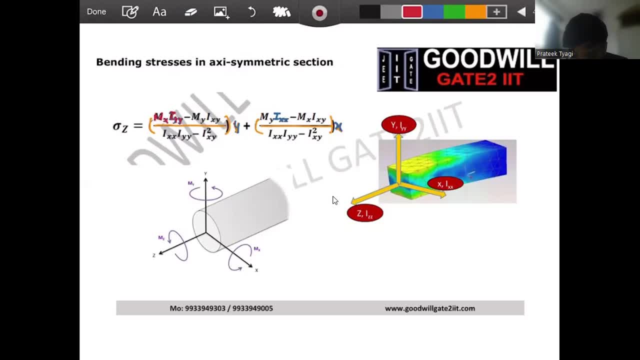 then you write opposite moment: MX here, you have written IXS, so you have written MY minus in both. If MX is covered, my will come here, my is present, mx is come here and then you have ixy. Anyhow, we will learn this formula when we start solving numericals. 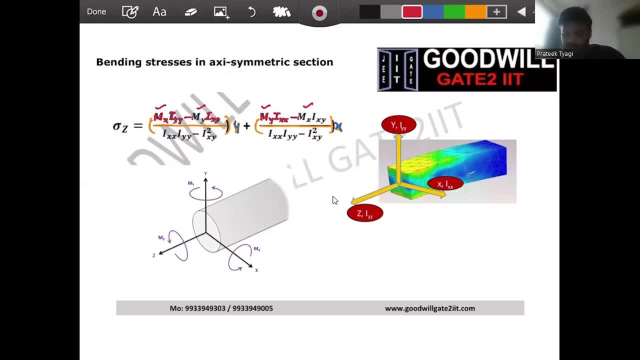 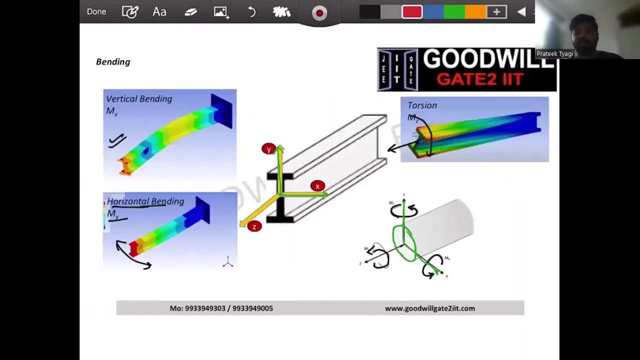 and, but you will see why this formula is in this form in just maybe next two, three minutes. Now, what this equation explains you and second, what is the meaning of this axisymmetric section? Now, please listen to me very carefully. If- and I want you people to answer this- I want you people to give it a try. answer my question. 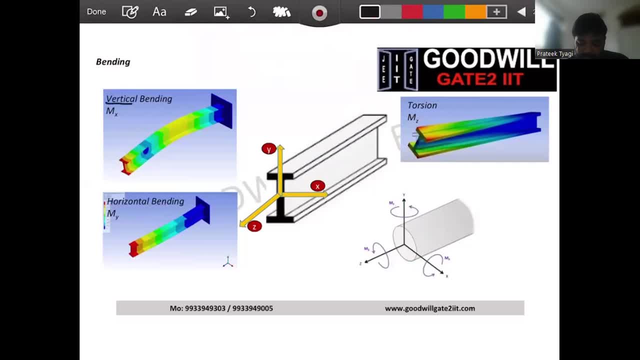 If you want your beam to bend in vertical plane- although I have written it here, the movement we want is mx. If you want your beam to go up and down, if you want your beam to go in horizontal plane, the movement we want is mx. If you want your beam to go in horizontal plane, the movement. 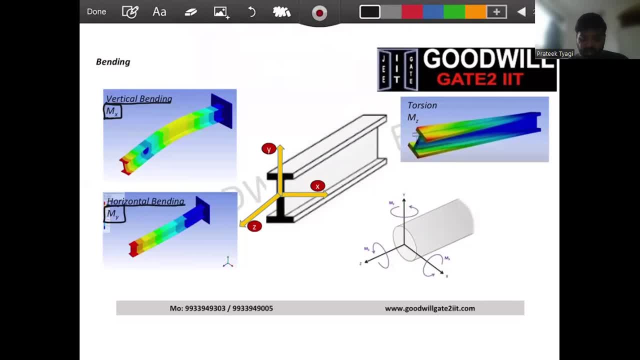 you apply is my. My question is if I apply both movements together. so, guys, this is only mx. if it is only mx, your beam will go up and down, Only mx. that means my is zero. no one is forcing it to go left and right. When you see this, this is my only, and mx is zero means it will go left. 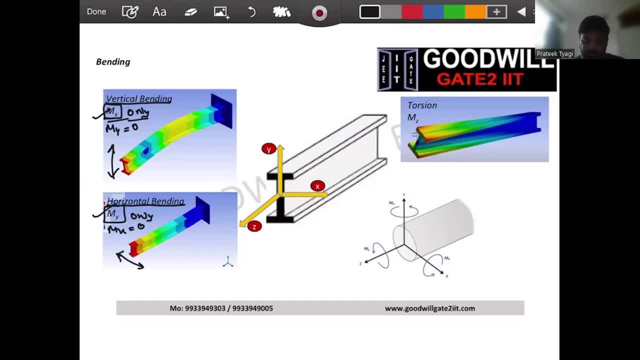 and right. My мой is mx. My question is if I apply both movements together- so this is only mx- if I apply the estoic right and before view, At this time, only my beam is moving up and down, My one is telling it to go up and down. but if you do both these things together, 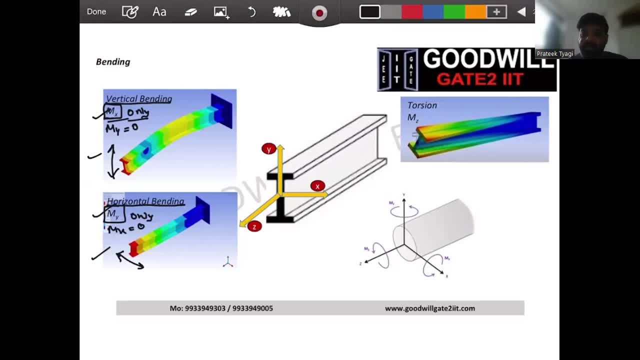 that means you apply horizontal bending also and you apply a vertical bending also together in one shot. now my question to you people is: you have applied both MX and my. what you expect your beam will go up and down, guys, or your beam will go left and right, or something else. what you people expect. 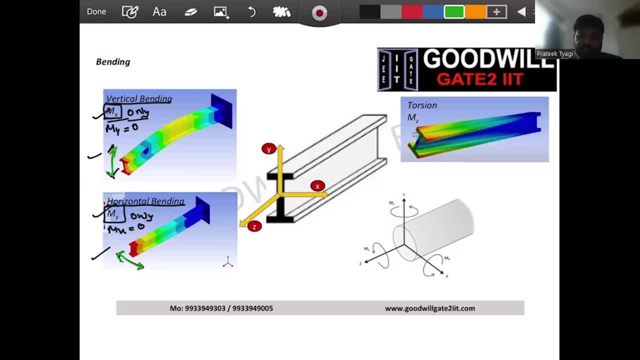 okay, good, good, good, Archisman. Archisman told me that it will be inclined. that's perfect. now, what do you mean by this? the meaning of this is: in diagonal XY plane perfection. so meaning your beam will try to go up and down, but it will also try. 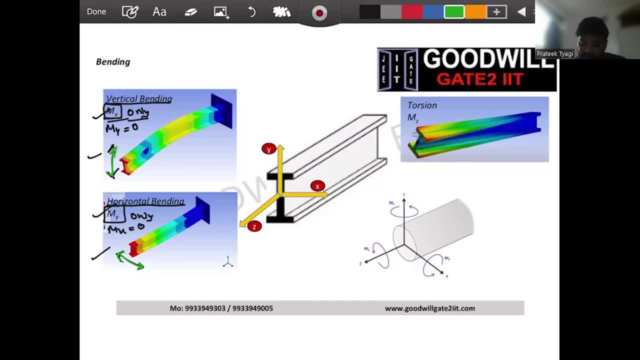 to go left and right, meaning maybe it will bend something like this, I hope you, I'm just giving you an example- so it will not bend only up down, it will not bend only horizontal, but because you have both the people pushing sidewards and upward, downward, you have 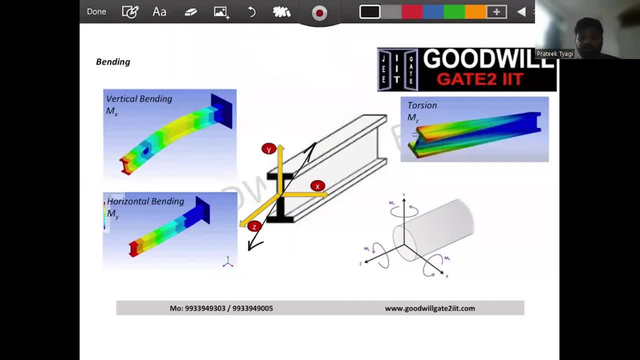 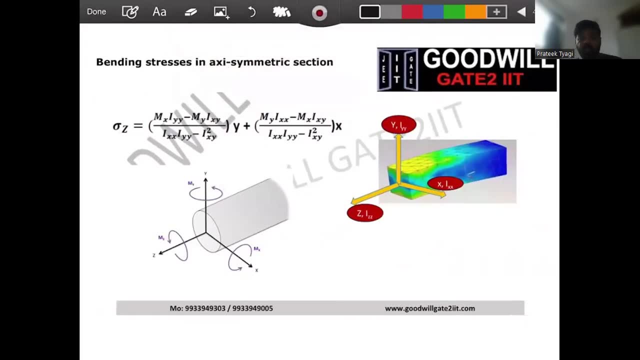 bending, maybe at some plane. this bending, which is not only in vertical and not only in horizontal, but in some other plane- some other plane means some inclined plane- is known as unsymmetrical bending. sometimes people also say this as asymmetric bending. so what is unsymmetrical bending, guys? a bending. 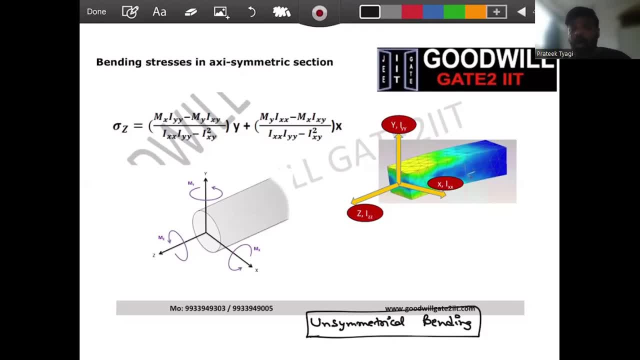 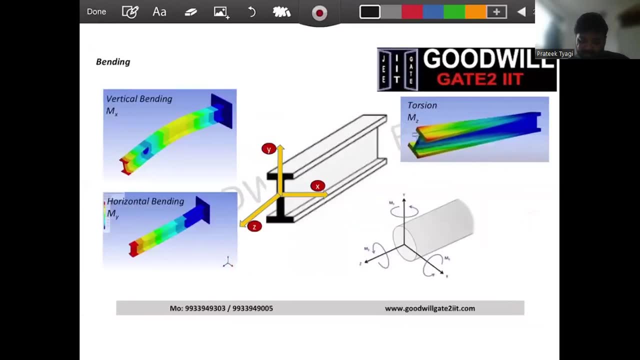 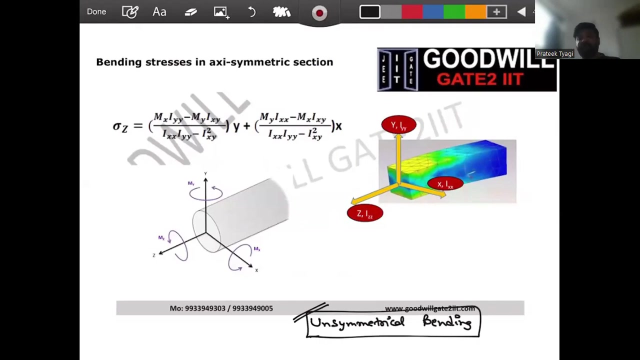 which happens in a combination of two planes or in an inclined plane. so the best example of symmetrical bending is: yes, this is symmetrical in vertical plane, this is symmetrical in horizontal plane, and if you go in some other plane, it is known as unsymmetrical bending. so from now on, if anyone guys, this is one. 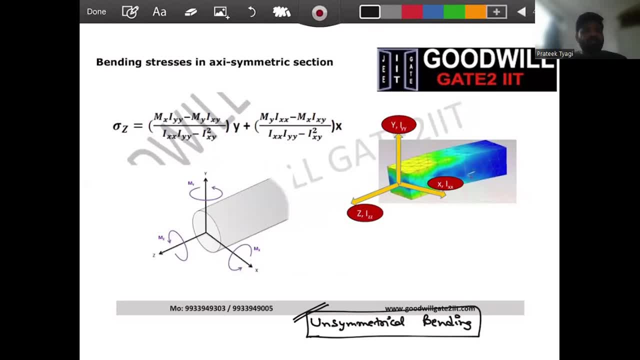 very common question asked in interviews. so if one asks you what is the difference between symmetrical and unsymmetrical bending, you directly say: unsymmetrical bending means unsymmetrical bending occurs in some inclined plane. And what is symmetrical bending? If you 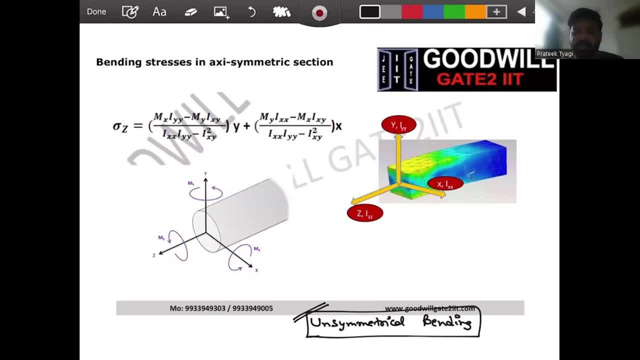 have pure vertical or you have pure horizontal, either one of them. both are known as symmetrical bending. Give me a quick nod. if this is clear to all of you, then I will go further into equations. Is this part clear to all of you? 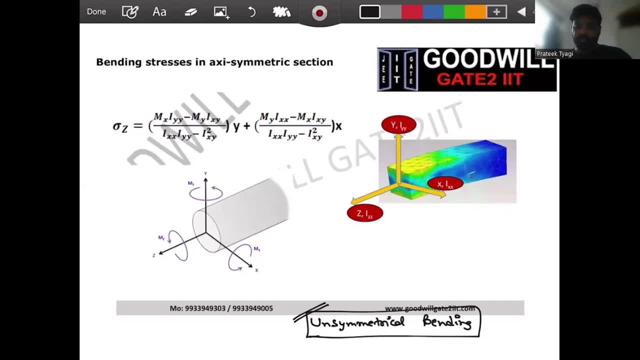 Perfect, Good, good, good. Now the next thing I want you people to understand is, although I will calculate for all cross-sections, but please take this as a note for time being, If you have any cross-section which is symmetric, all right. now, please listen to me very carefully- Any cross-section. 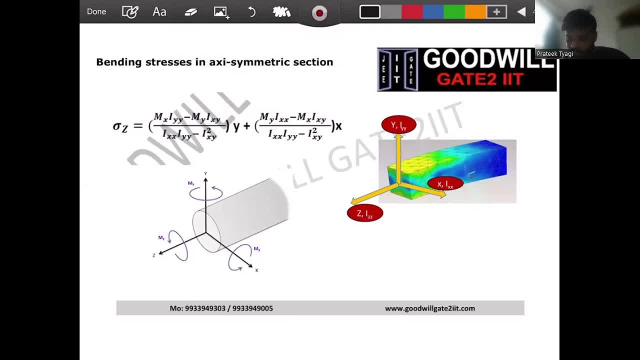 which is symmetric now please listen to me very carefully- Any cross-section which is symmetric. now what is symmetric cross-section? A rectangle is symmetric about this axis: right. Symmetric means left and right is same, And rectangle is also symmetric about this axis means up and down. 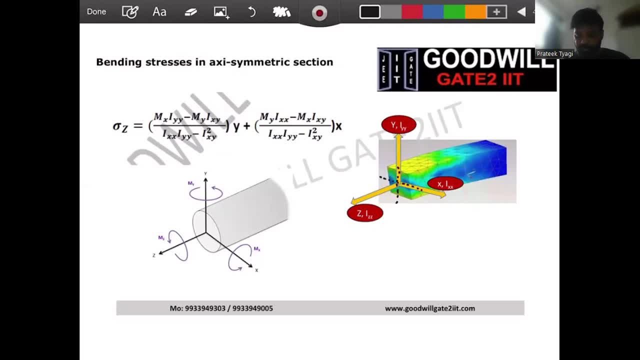 is same. You can easily imagine the word symmetric, right. So this is a double symmetric cross-section. Rectangle is a double symmetric. X-axis is also symmetric, Y-axis is also symmetric. Similarly, if you see circle, if you cut, you have two similar. 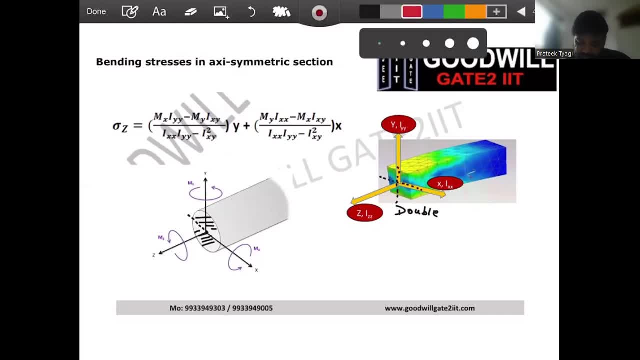 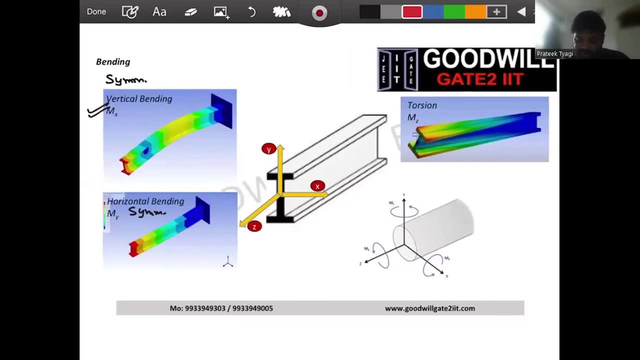 this is symmetric And if you cut it vertically it is also symmetric, So this is also symmetric. cross-section. If you see I-section, this I-section is symmetric about Y-axis- left and right are mirror image- And this I-section is also symmetric about X-axis. that means top and 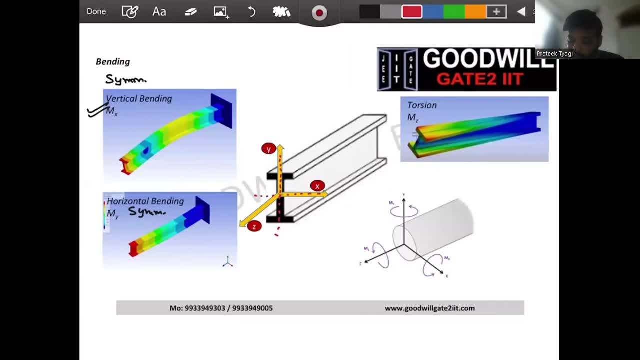 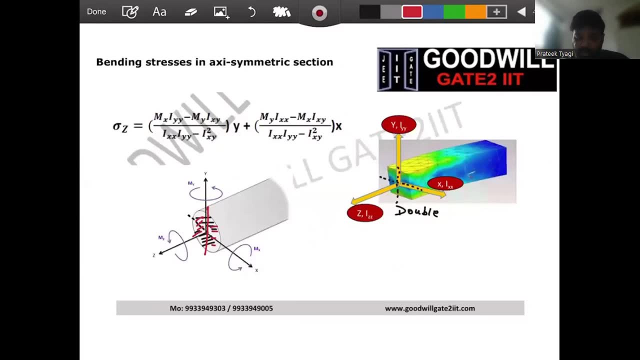 bottom are also same. Now what I'm trying to portray here. I will show you this slowly, because I have all the slides for calculating inertias. But what? just as of now, please remember this- When your cross-section is symmetric, all right, whether it is single symmetric or doubly. 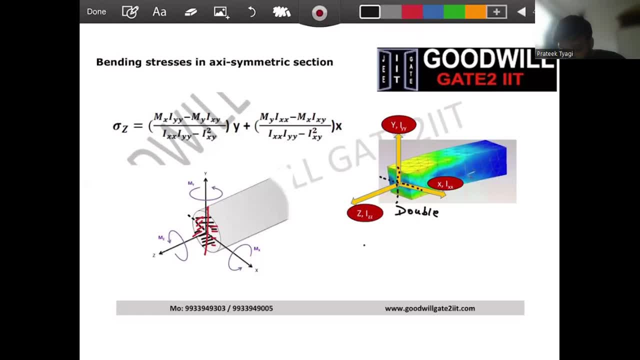 symmetric. Now I'll give you an example. If you see C-section, this C-section is symmetric about only X-axis. You see, top surface and bottom surface are exactly same. So it is symmetric about X-axis, but it is not.